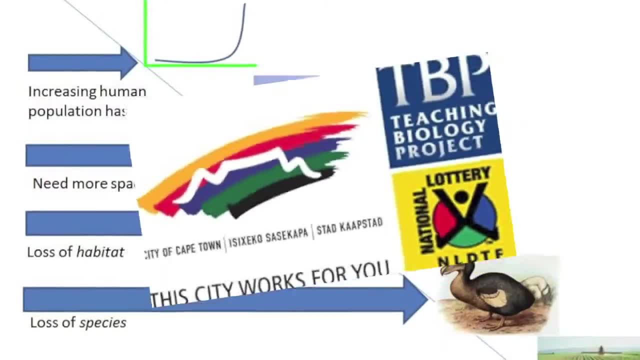 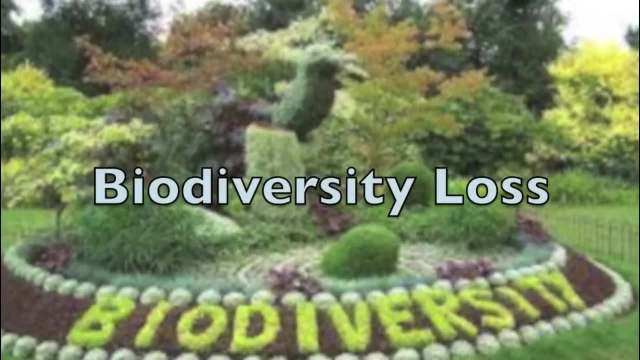 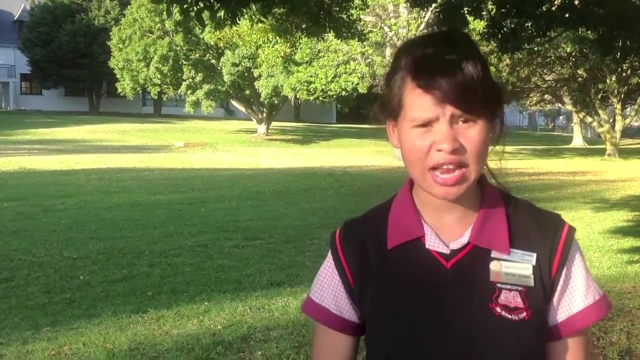 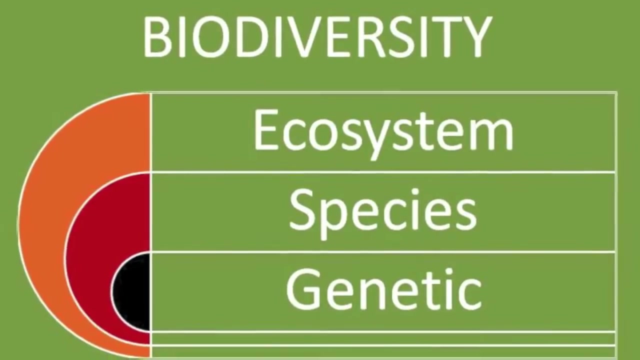 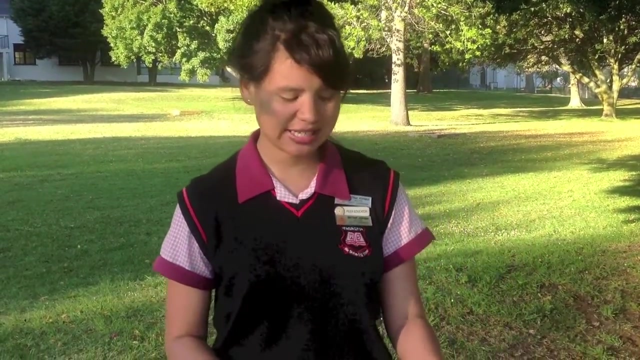 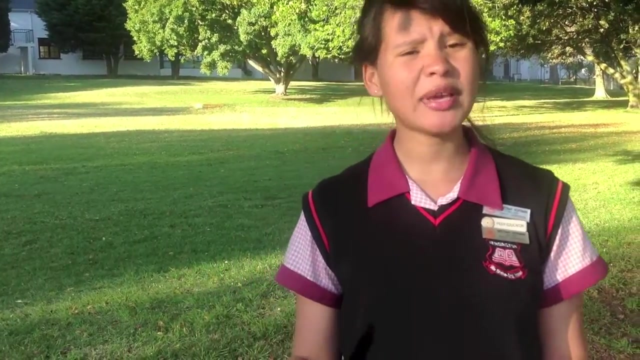 What is biodiversity? Biodiversity is the variety of living organisms. There are three important aspects to biodiversity. Number one: ecosystem diversity. This is the variety of habitats available for different species to live in. Number two: genetic diversity: The variety of characteristics found within a particular species. Number three is species diversity. 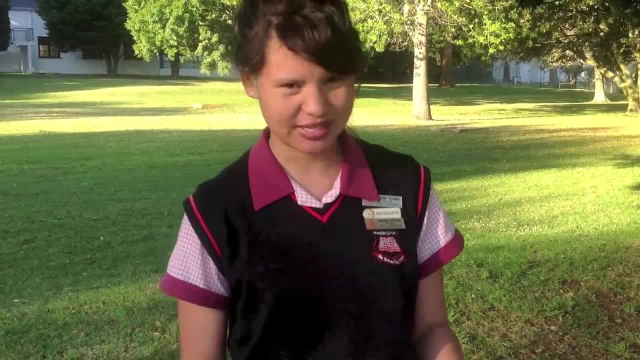 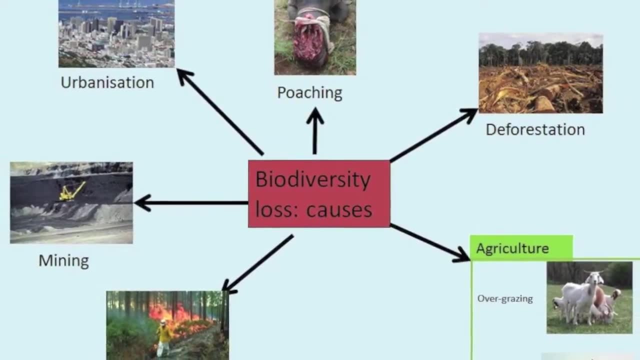 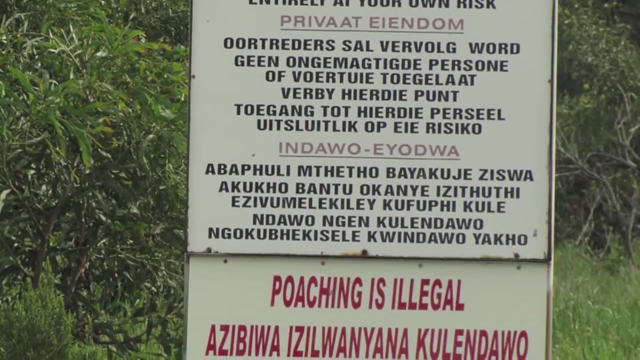 The variety of different species found within an ecosystem. What is biodiversity? Urbanization? This alters the very surface of the land. This includes the roads, the buildings, the concrete, the gardening, poaching, which is the legal taking of wildlife. This includes rhino poaching and parallel moon. Deforestation is the clearing. 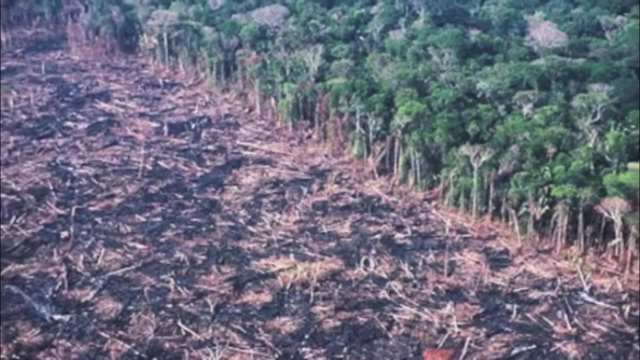 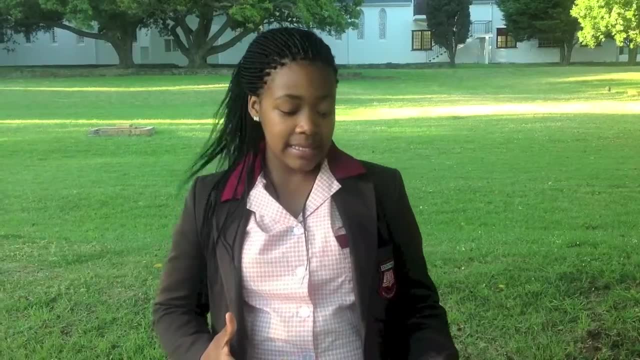 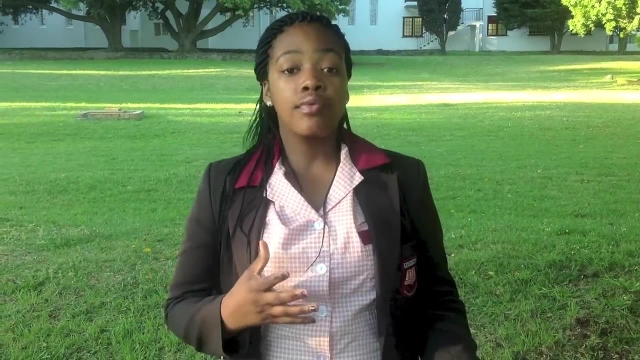 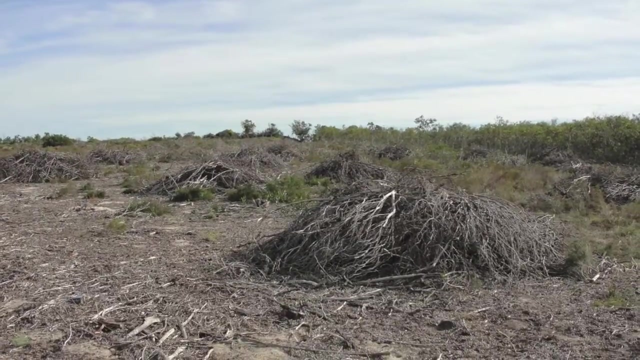 of flora so that land can be used for urban development and agriculture. Invasive alien species: There are species that have been introduced into an area where they don't belong and therefore have no natural predators to control the population size. As a result, they have overpopulated and dominate our indigenous species. Why is Cape Town so special? 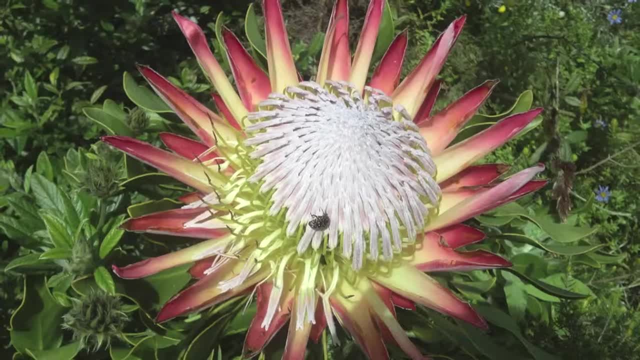 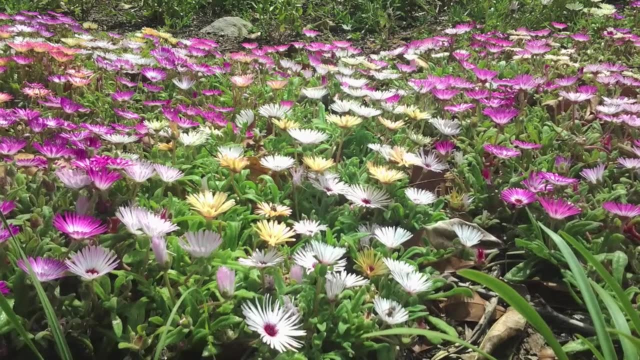 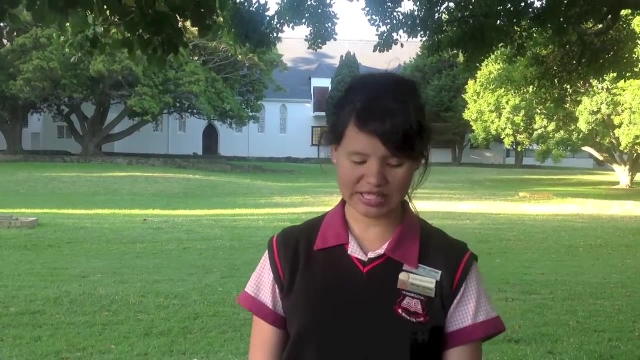 in terms of biodiversity. South Africa is home to the Cape Florida Kingdom and is the smallest of six and one with the highest density of plant species. Cape Town is situated in the heart of the Cape Florida Kingdom, making the area important in a global aspect. Cape Town consists of many endemic. species, meaning the species are truly and only found in this particular area. Cape Town contains 19 vegetation types. It all belongs to the highest threat class, which are critically endangered. Cape Town is home to 50% of the country's threatened ecosystems, Having 318 threatened. 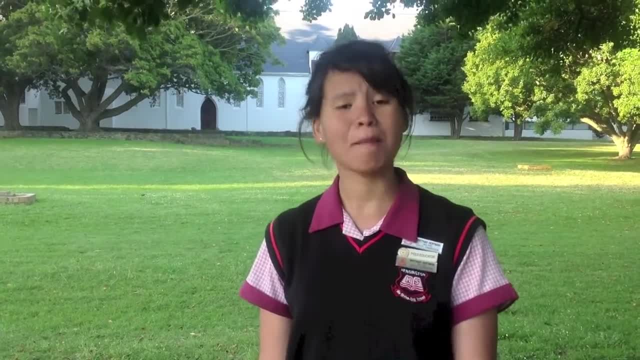 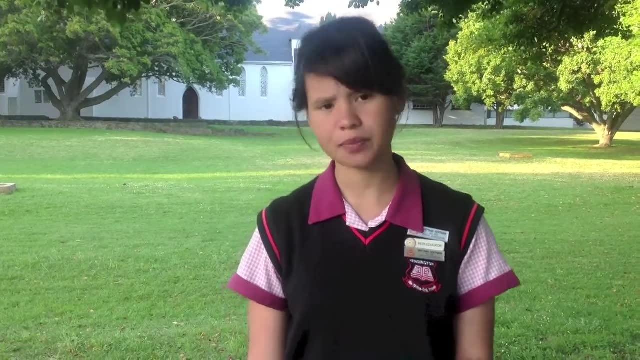 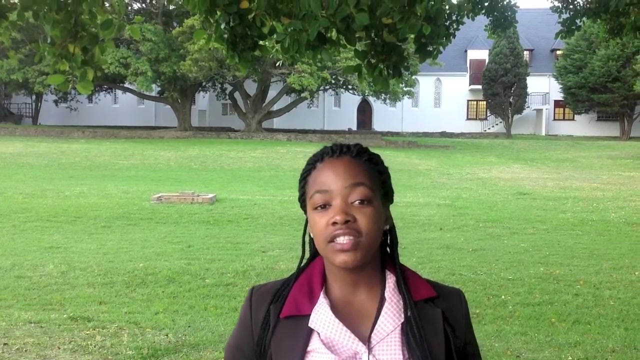 plant species and known as one of the Earth's mega-seas disaster areas, which are on the verge of losing a significant part of biodiversity. The value of biodiversity. Biodiversity performs a number of ecological services for humankind that have economic and recreational value. 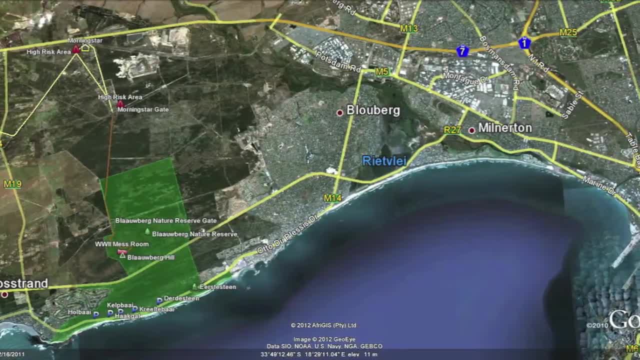 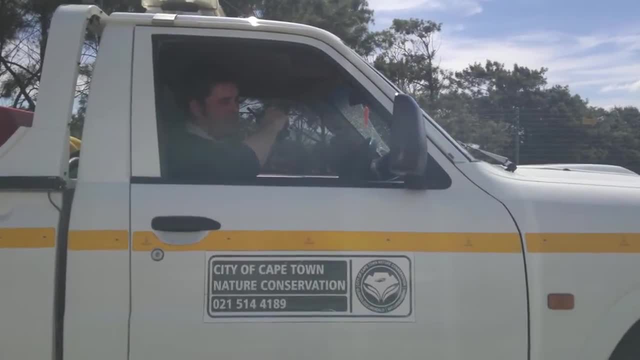 Threats that Bloberg is faced with. Urbanization affects the biodiversity at Bloberg Nature Reserve in a sense that people build infrastructures- schools, hospitals, houses, etc. And through this development there is a demand for space And the spaces which are used to build infrastructure. 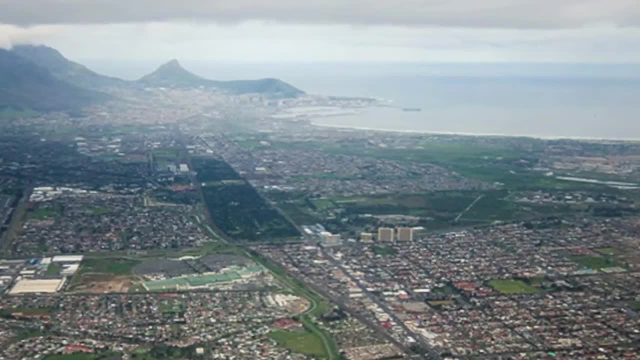 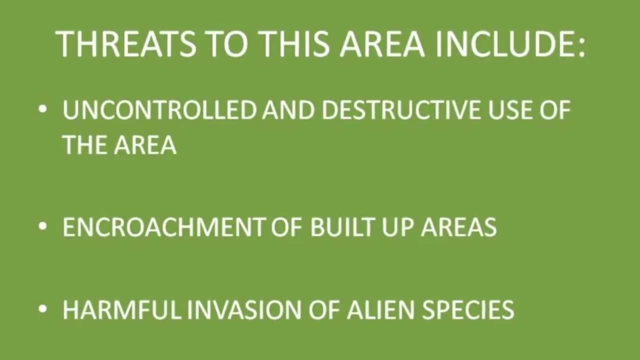 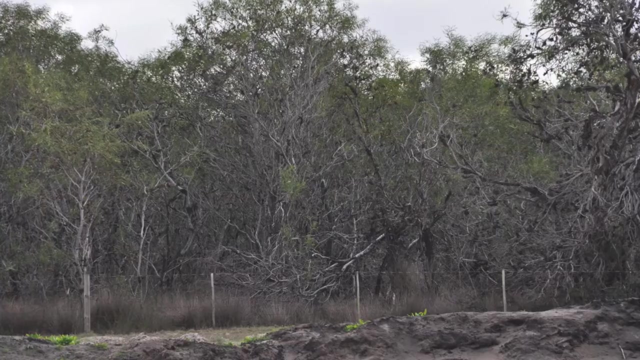 which is mostly desired for, is already occupied by a variety of plant and animal species. Invasive alien species are one of the major threats to biodiversity at Bloberg. They consume large amounts of water. For example, the Port Jackson consumes 1000 litres of water on average. 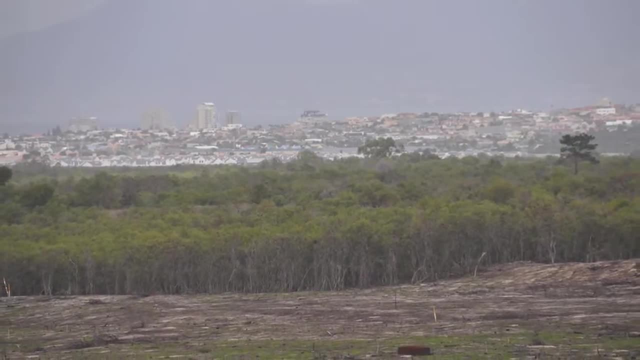 per day, And this poses a great threat to our water security. Alien plants which invade the area do not have the natural predators and therefore overpower the natural environment. In addition to this, there is also a great threat to our water security. Alien plants. 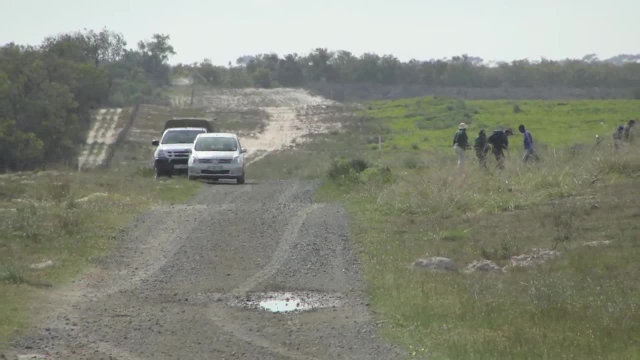 which invade the area do not have the natural predators and therefore overpower the natural environment. In addition to this, there is also a great threat to our water security: Alien plants which invade the area do not have the natural predators and therefore overpower the natural environment. 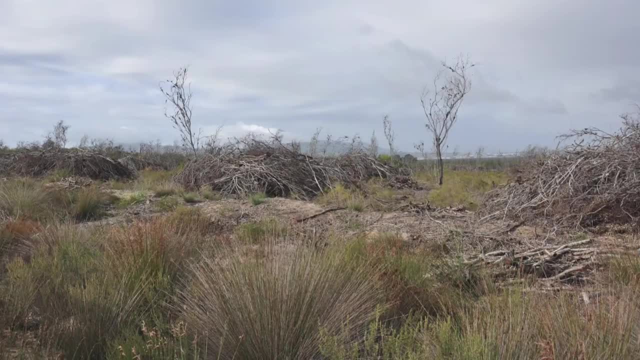 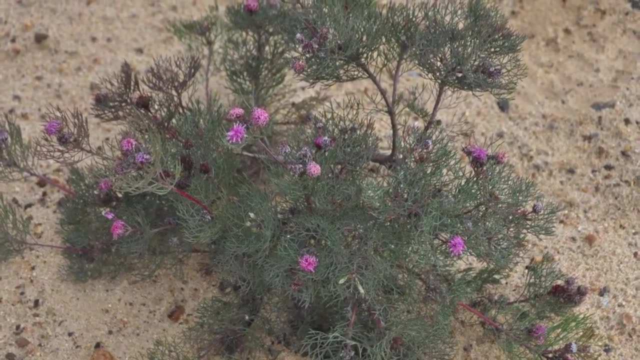 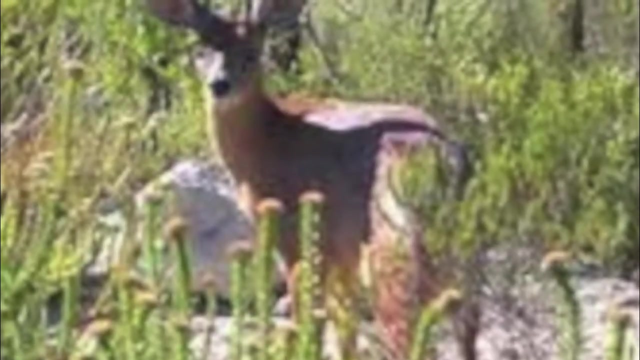 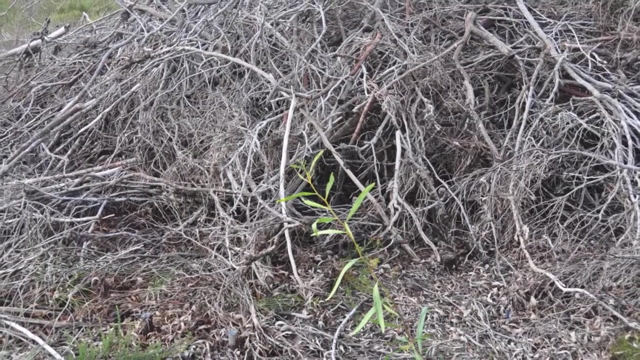 This also results in denomination of indigenous species. Test passing threatens biodiversity and people who tread over plants and therefore damage the plants and also scare of animals that occupy the area and damage their habitat. Plants are also being put in place to protect the flora and fauna of our country from being harmed by man. Alien invasive species are being cut down. 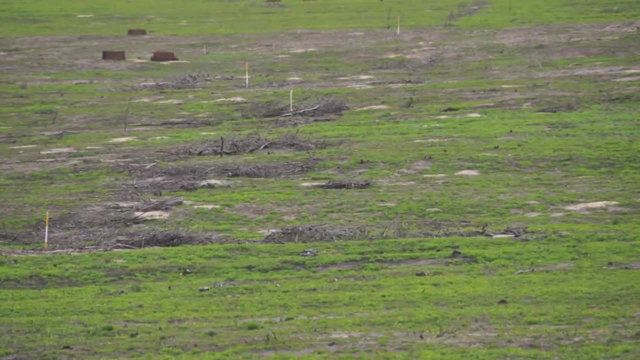 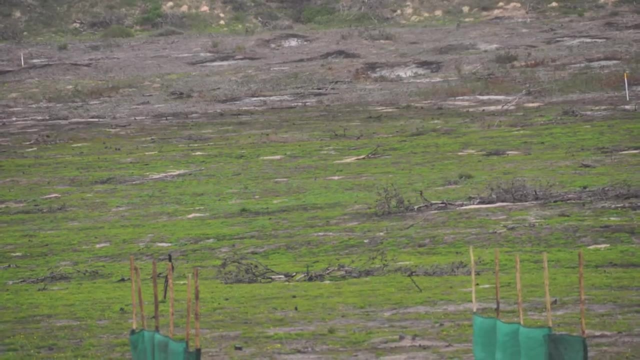 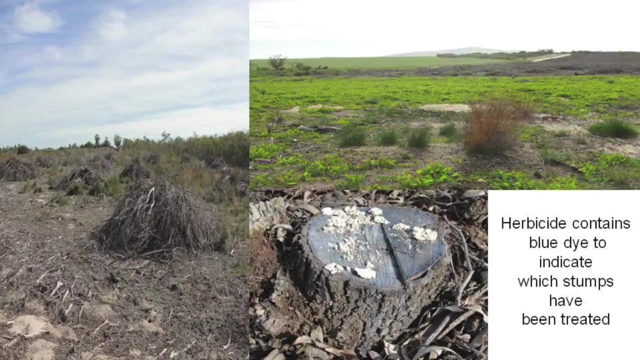 stacked in piles and then are burned up. The remaining tree stacks are then sprayed with herbicides to prevent it from regrowing. These herbicides contain a blue dye which acts as a marker. This is being done to provide more space for the indigenous species to be planted. We have decided that the most suitable solution. 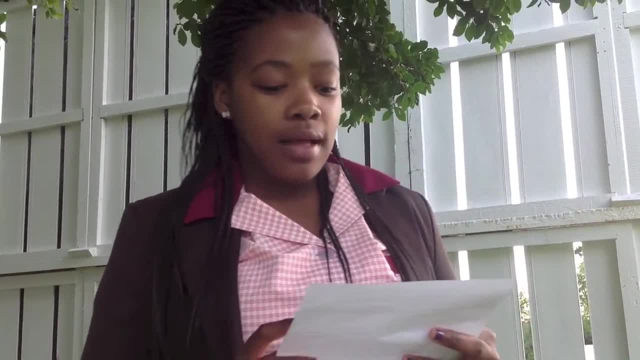 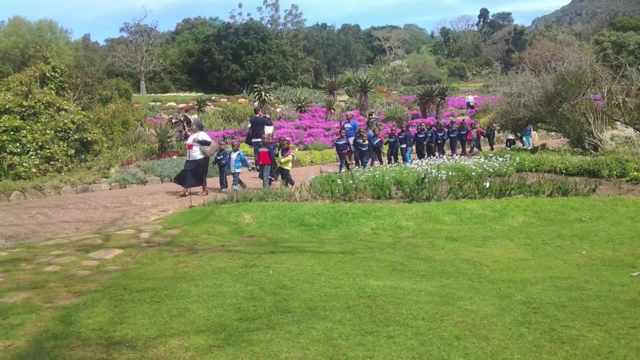 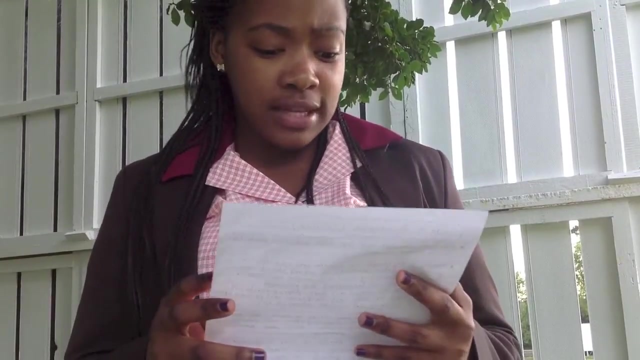 is to create awareness. We, as young people, can inform and educate our peers and fellow students at school about the matter and create awareness and, as soon we can, broadcast the message throughout the school and thereafter, parents will know about this issue and companies and organizations will be informed and will. 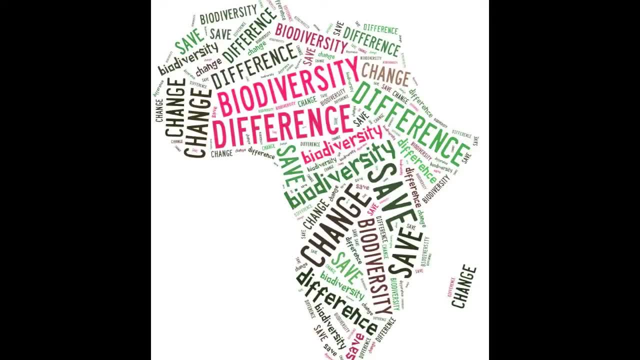 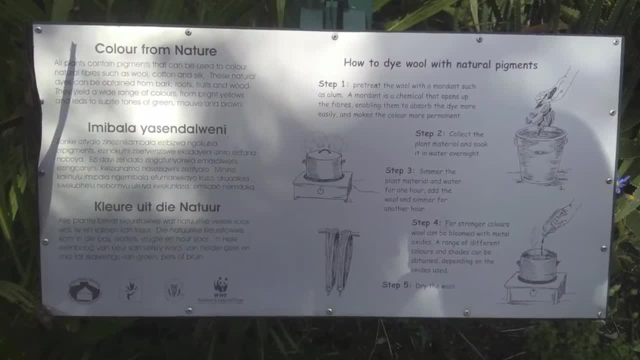 take action as well. We can go to public areas and set up posters and give up pamphlets to educate and create awareness of biodiversity loss and even promote indigenous gardening. There are many ways to promote indigenous gardening. There are many ways to promote indigenous gardening.